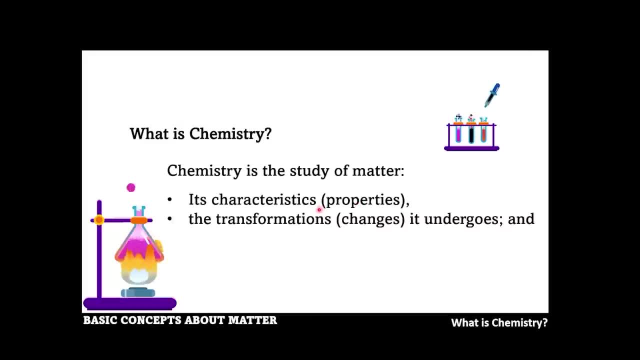 be physical properties or chemical properties. It involves study of transformation, which can be change- it can be physical change or chemical change- and study of energy associated with the changes, whether it is losing energy to the environment or it is gaining energy from the environment. Therefore, all these areas must be considered during the study of matter. 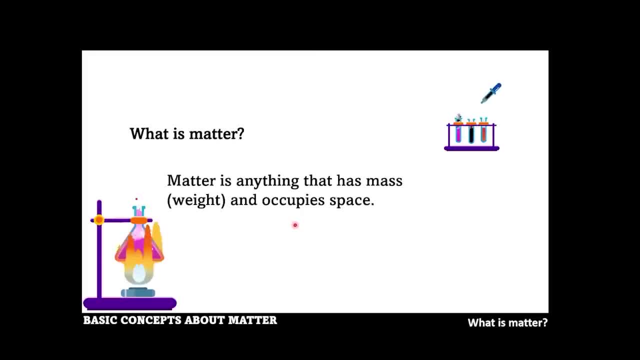 Let us look at matter. Matter is anything that has weight and occupies space. As you are watching this video, there are a lot of items around you that you need to consider when you are studying the study of matter. There are a lot of items around you that can be classified as matter. Matter can be. 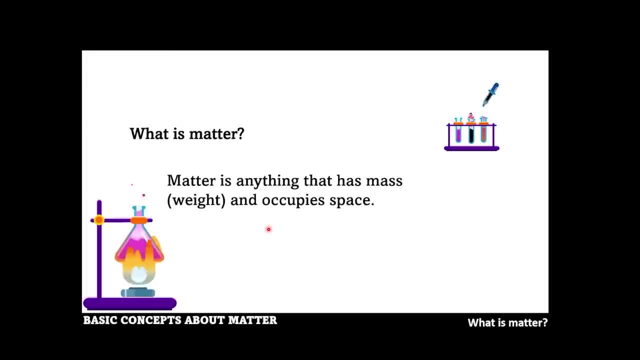 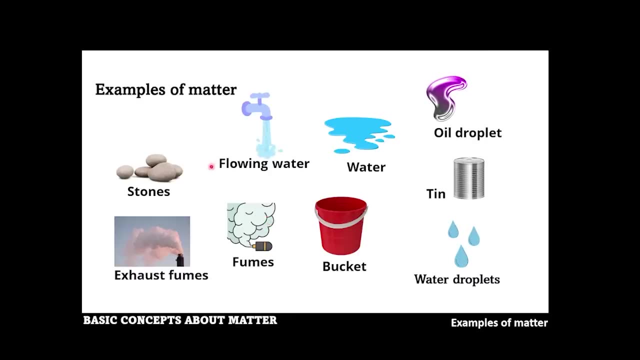 found around us. Your mobile phone is a matter. The cup beside you is a matter. The quantity of water to matter can be found around us and they are part of our daily life. Let us look at the following examples I listed to help our learning. 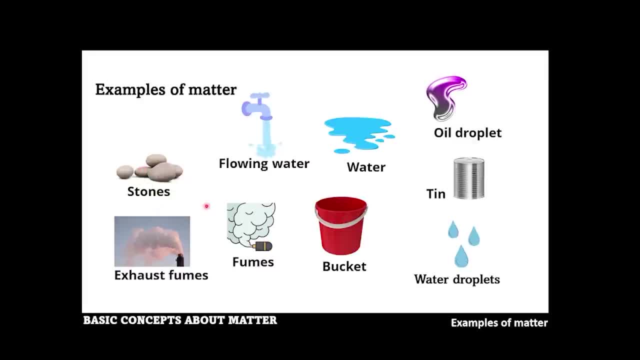 about matter. If you look at the following examples, they are not too difficult for us. The slide contains items we see in our daily activities. Stone can be found around us. Flowing water is not new to us. Fumes from the canister is not new to us. Bucket water: 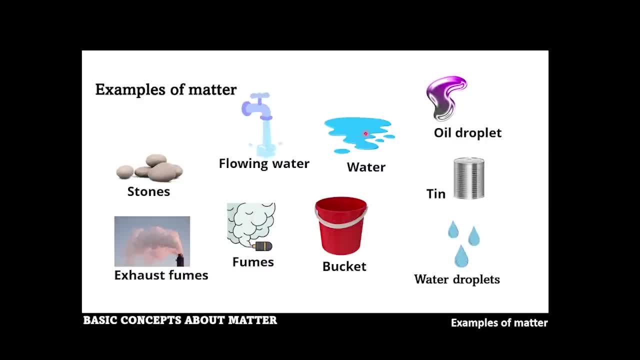 droplet water, spray on the ground and gas from the burning chamber are different examples that are not too difficult for us. One of the benefits of using the slide is that it can help us learn more about matter. Using these figures as examples is to help our learning, since a mental picture gives. 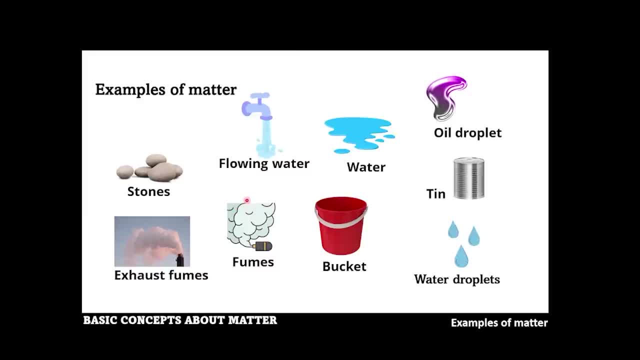 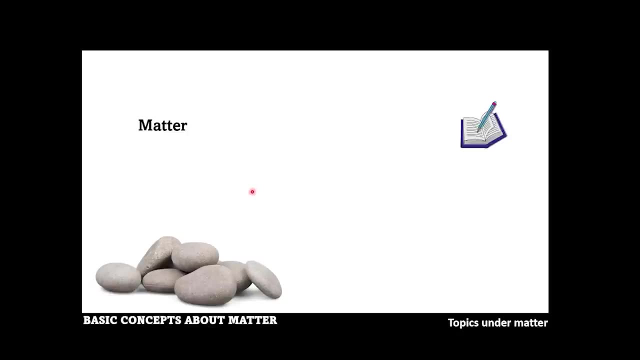 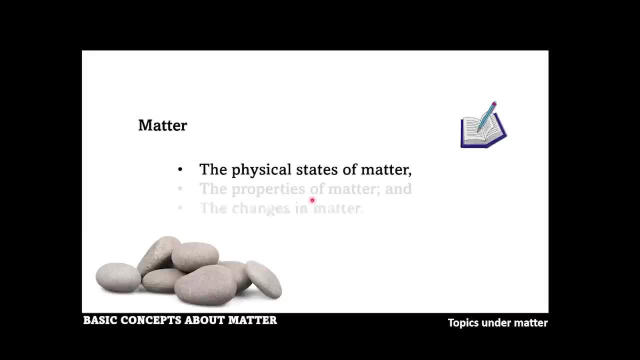 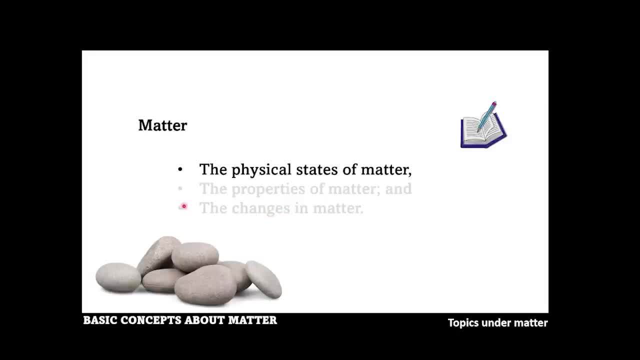 matter will help to classify those examples I showed in the last slide into various physical states. The example I showed in the previous slide can be categorized into different physical states of matter based on their properties. So there are three physical states of matter: solid, liquid and gas. Let us go back to those. 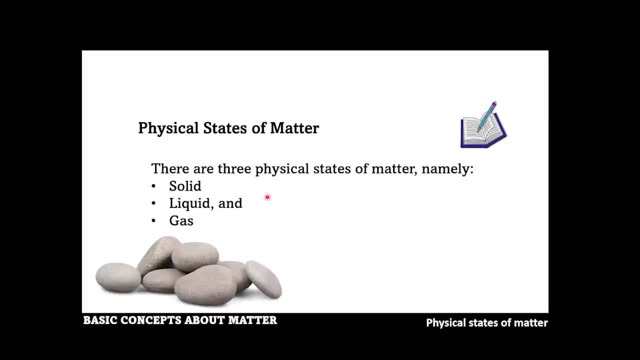 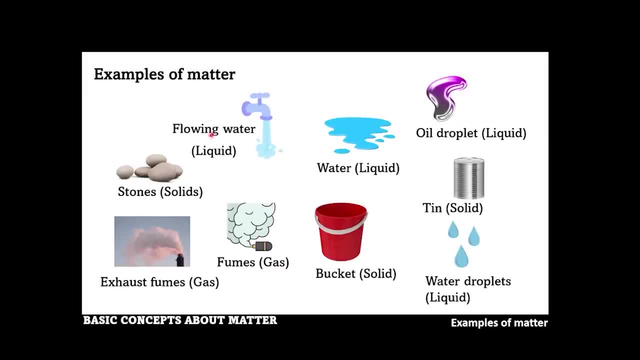 examples and see how each of those items is categorized into different physical states of matter. As you can see, stones are solids, Flowing water is liquid. Oil droplet is liquid. Bucket is solid. Water droplet is liquid. I want you to know that at times, an object may. 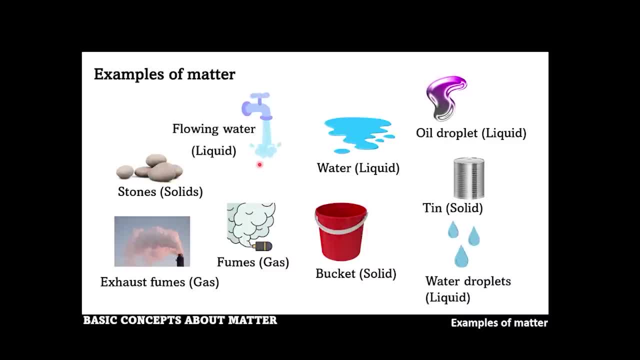 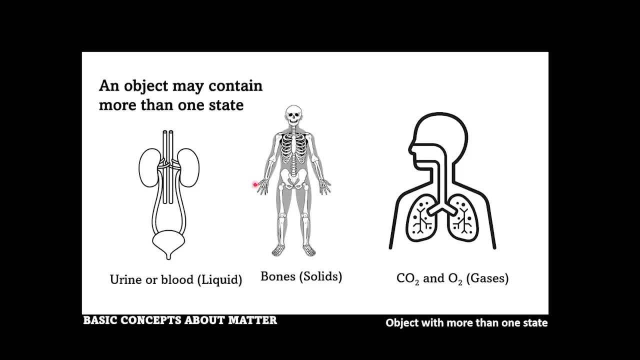 contain more than one state of matter. For instance, human beings like you and I comprises of three states of matter. Let me give you an example. As you can see, the following systems in human body, Urine or liquid portion of blood in our system, is liquid. 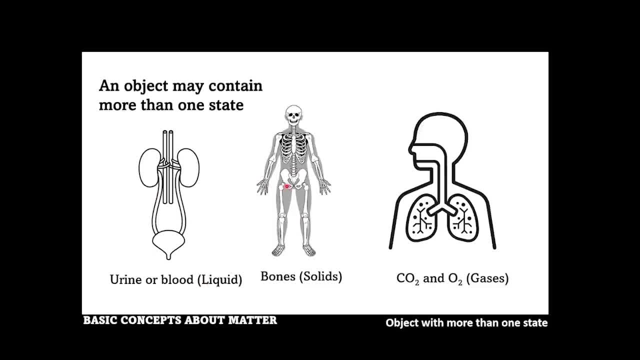 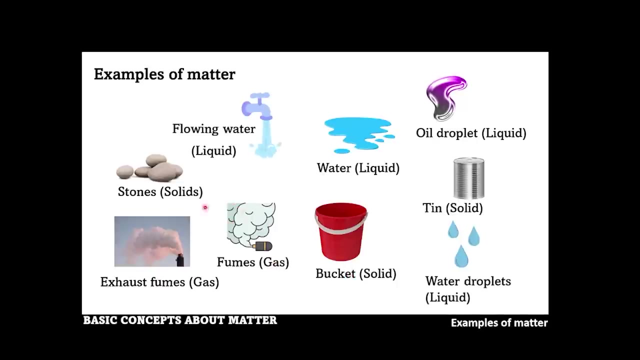 Bones in our body can be classified as solids. Oxygen and carbon 4 oxygase exchange during the blending process are gases, So it is possible to have an object with more than one physical state of matter. Let us look at the properties or characteristics I use to classify each item as either solid. 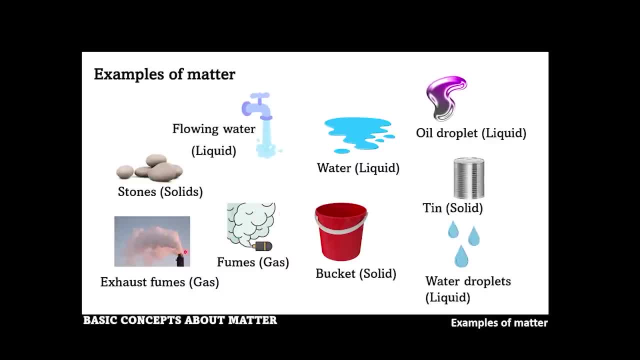 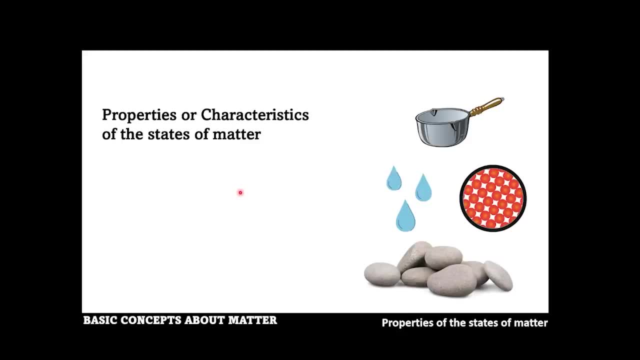 liquid or gas. It will explain why these items are classified as liquid, solid or gas. The properties used include shape, volume, relationship with a container, cohesion force and compressibility. I will discuss each state in detail using these properties or characteristics. Let us consider: 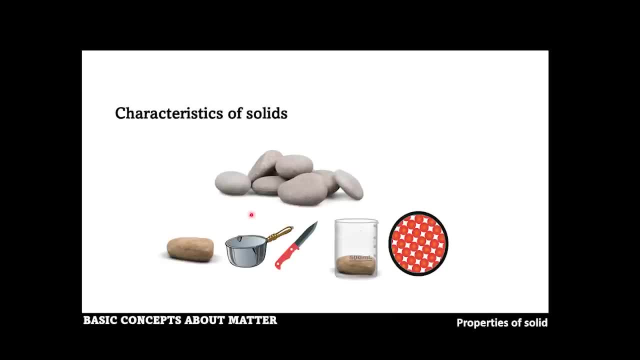 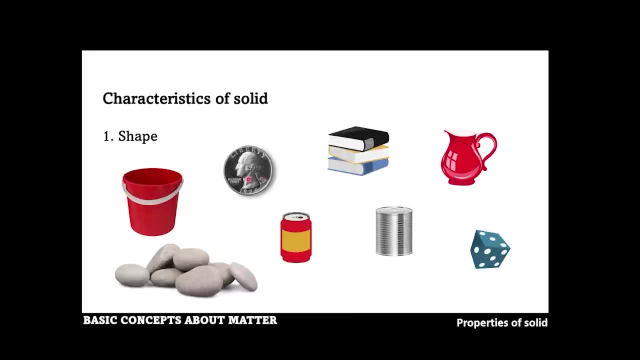 the following. Let us consider the following. Let us consider the following. Let us consider the criteria of solids Shape. Looking at the shapes of all items in this slide, The best way I can explain this is that in the next 5 years, do you think the shape of the following solid objects will? 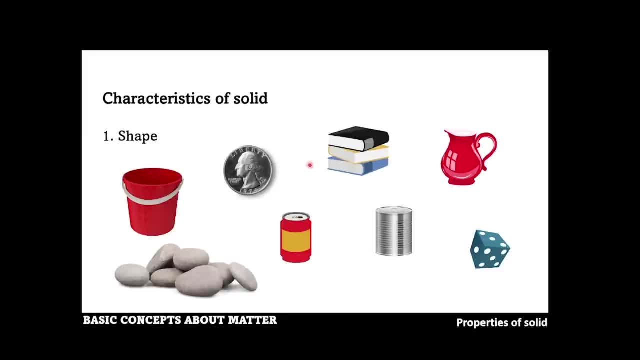 change, if not external force changes their physical appearance. Answer is no. the object will remain in the same spot, will remain in the same size, in the same shape in the next five years if nothing happens to them. So in that case we can conclude that solid. 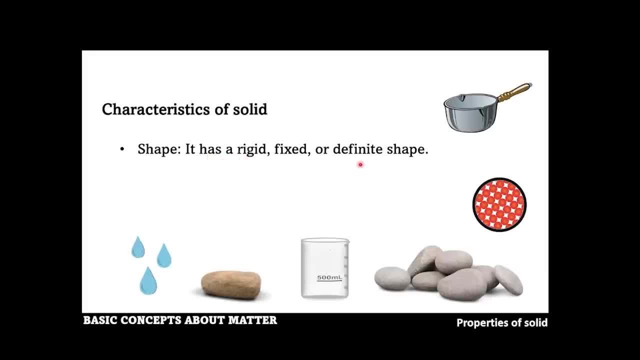 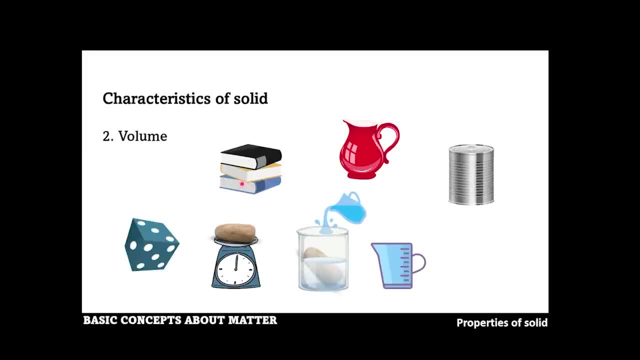 has a rigid, fixed or definite shape In terms of volume. solid objects can be regular or irregular objects. Regular objects have regular dimensions. therefore, regular objects can be measured with simple methods like using a ruler or through mathematical formulas, For instance the volume. 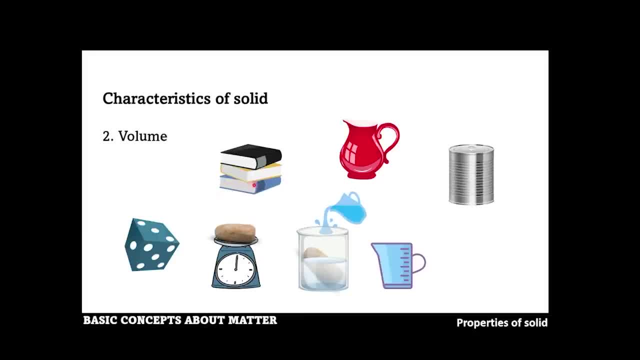 of rectangular shape, which is the shape of a book, is length multiplied by the breadth multiplied by the height. It can also be applied to the die. For the shape of a book, it is the length multiplied by the breadth multiplied by the height. For the 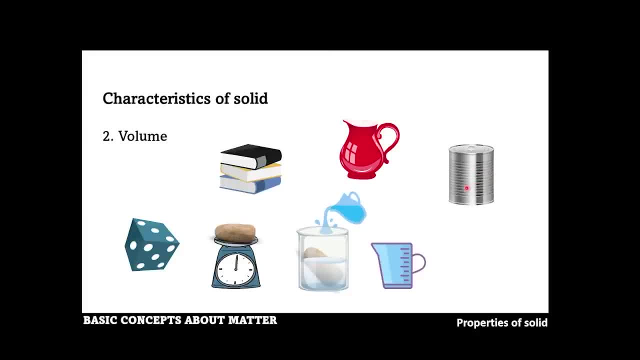 cylinder. it can be pi, r, square h, with radius and height as variables. How can the volume of an irregular object like stone be estimated? The volume of stone can be estimated using Archimedes' principal emphasis. However, irrespective of the method used to estimate the volume of solid, if the volume 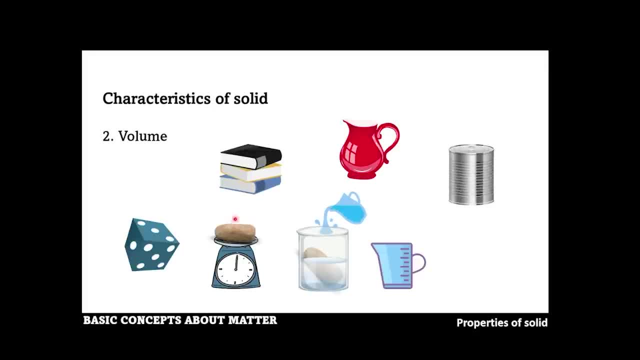 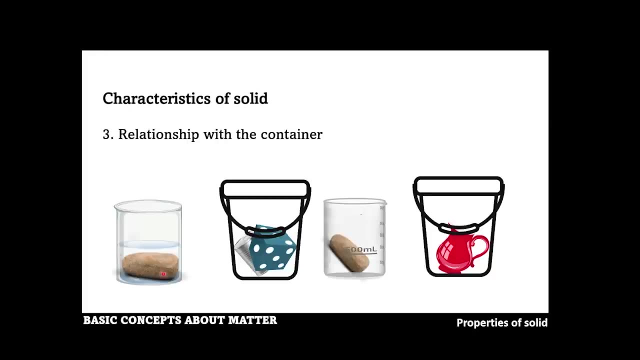 of the solid is measured for different times, like today, 5 days time, 10 days time, 5 months, the volume remains the same. In that case, we can conclude that solid has a definite volume. Let us consider the relationship of solid with the containers. 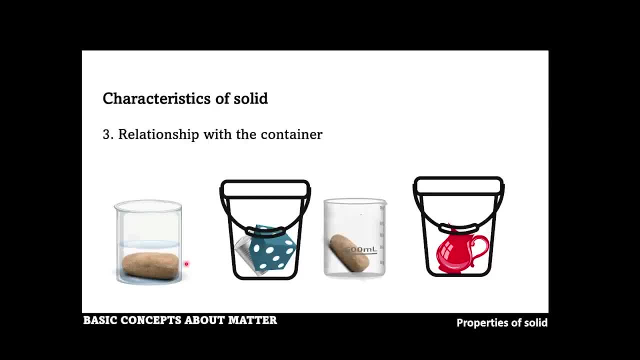 Considering these solids inside these containers. do you think these solids inside the containers lose their shape? The answer is no. The solids still maintain their shapes because the containers do not detect or affect the original shape of the solid. Therefore, we can conclude that solid does not take the shape of the container. 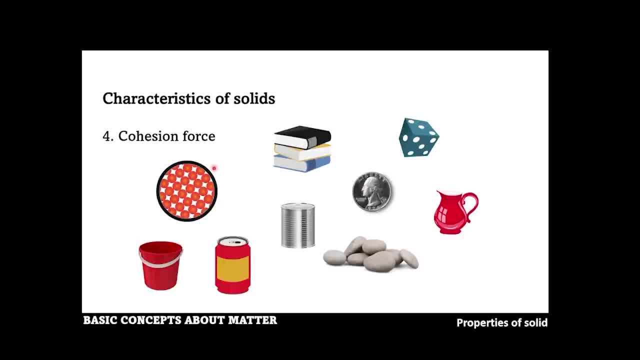 The next property is what is called coercion force. The best way to understand coercion force is to understand the following: The first property of coercion force is to use the particles arrangement in solid, which is shown here. As you can see on the slide, solid particles are closely bonded together. 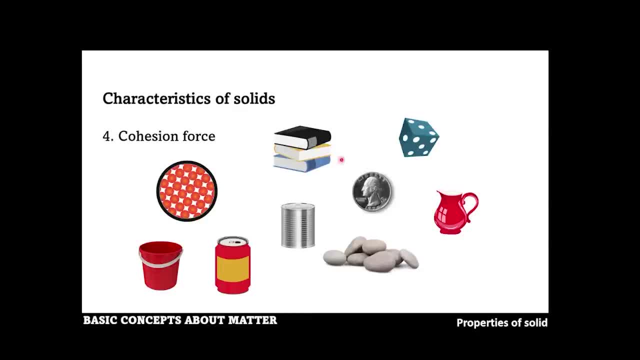 Because they are bonded together, they are responsible for the properties of solids. The particles are closely packed due to the strong force of attraction between these particles. So when you look at the particles arrangement, you can see that solid particles are closely bonded together. 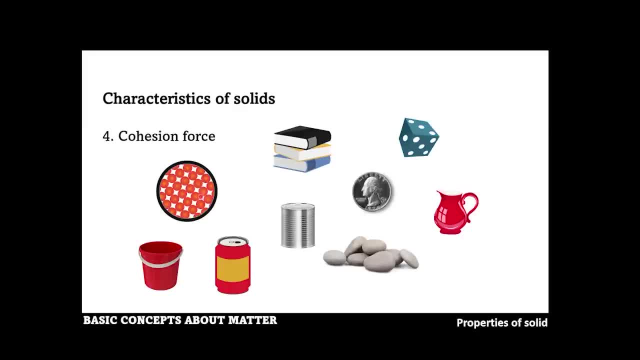 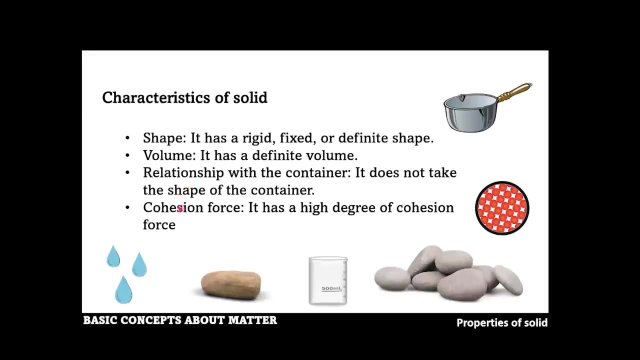 But when you look at the particles, there is no free space in between these particles. One particle cannot easily displace another particle And because of this solid has a high degree of coercion force. So the conclusion is that solid has a high degree of coercion force. 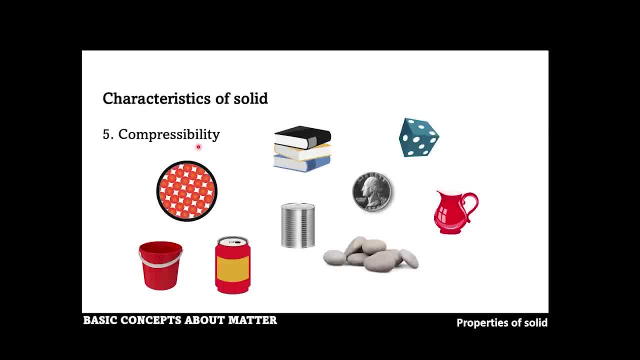 The last property to consider under solid is what is called compressibility. It can also be explained using the particle arrangement. You cannot compress the coin, You cannot compress the book, You cannot compress the die. They are challenging to compress because the particle's arrangement is closely packed together. 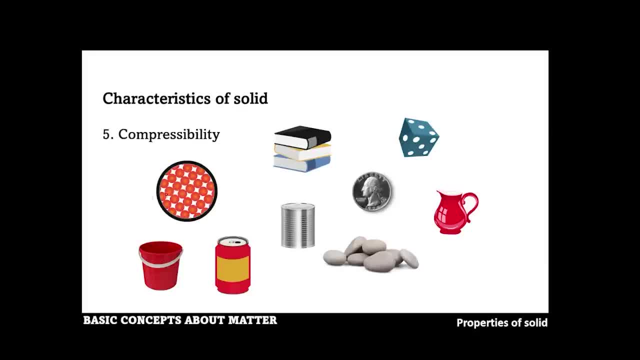 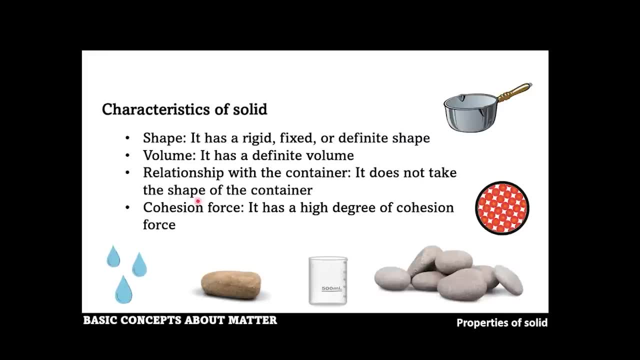 Each particle maintains its space, preventing displacement by another particle. There is no free space for movement. In conclusion, solid cannot be compressed. That completes the characteristics of solid We can see in terms of shape, volume, relationship with the container, coercion force and compressibility. 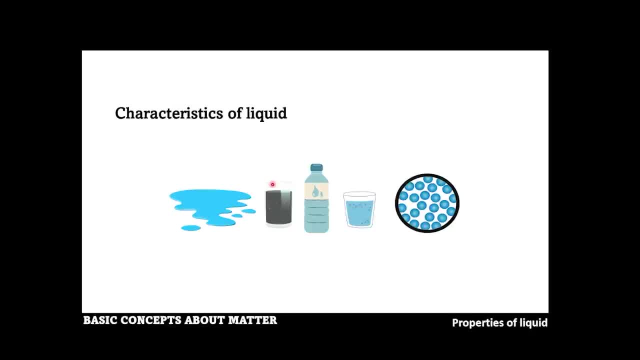 Let us consider the characteristics of liquid In terms of shape. suppose the same quantity of water is transferred from one container to another. You will notice the shape of the liquid changes. The liquid has a different shape when it is on the ground. It has a different shape when it is inside the bottle. 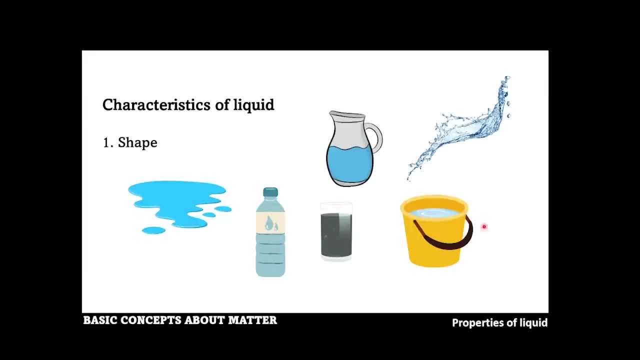 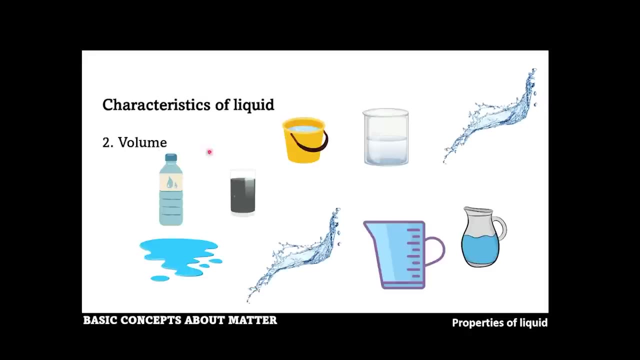 It has a different shape when it is inside the cup And it has a different shape inside the bucket, So the shape changes. So in that case we can conclude that the liquid has no rigid or definite shape In terms of volume. in the same way, let us assume the same quantity of liquid is measured. 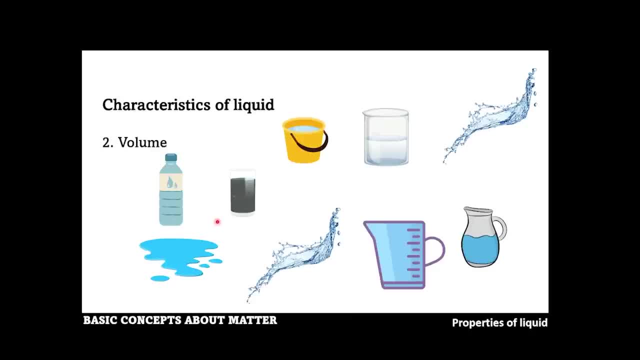 and transferred from one container to another. Then, provided there is no leakage, the same quantity is transferred to the cup, the same quantity transferred to the bottle and the same quantity transferred to the measuring cylinder, From there to the measuring cup, And so on. 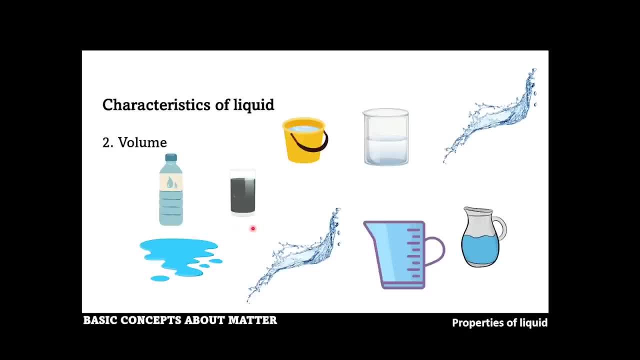 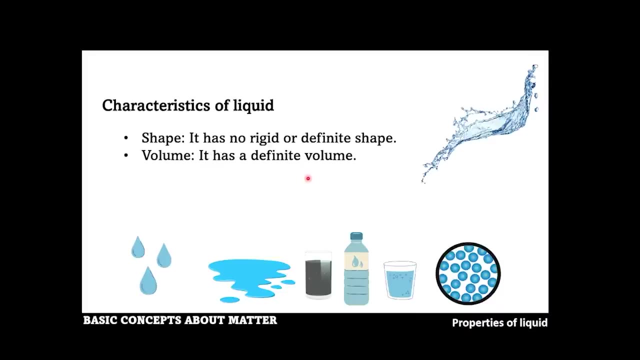 In that case, you will discover that the volume of liquid remains the same, because the quantity transferred from one container to another remains the same. Therefore, we can conclude that liquid has a definite volume. In the previous slide, I discussed the shape of the liquid. 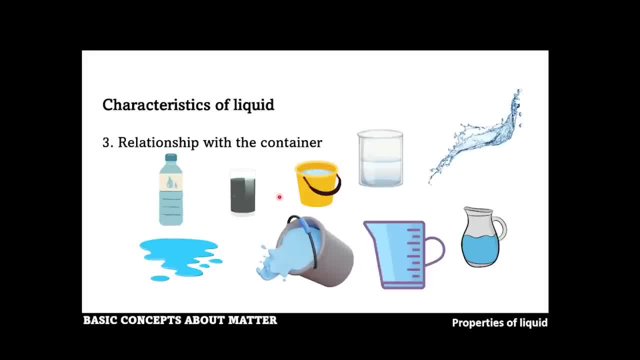 When the liquid is transferred from one container to another, you will notice that it takes the shape of the container. For example, the liquid has different shape on the floor, It has a different shape inside the bottle And it has a different shape inside the glass cup. 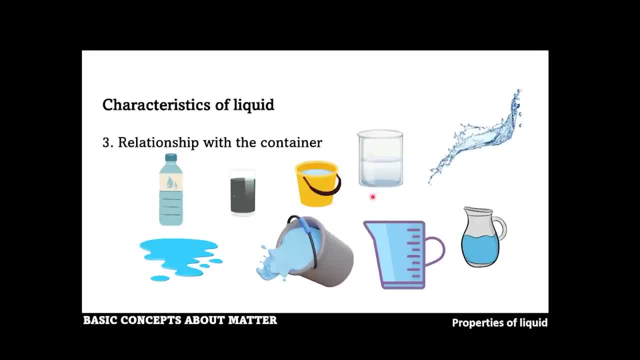 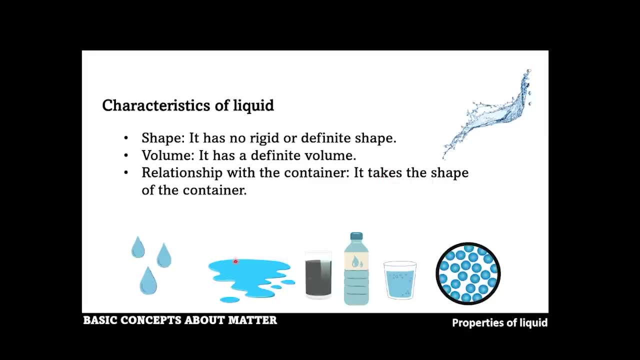 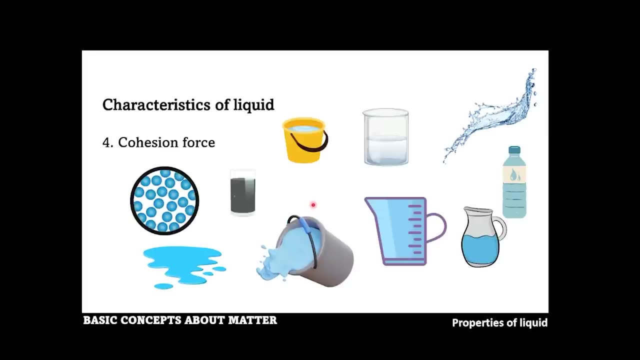 It has a different shape inside the bucket And it has a different shape inside the jug. We can conclude that liquid takes the shape of the container, Because the container dictates how the shape of the liquid will look. like Coercion force. To understand the coercion force, we still 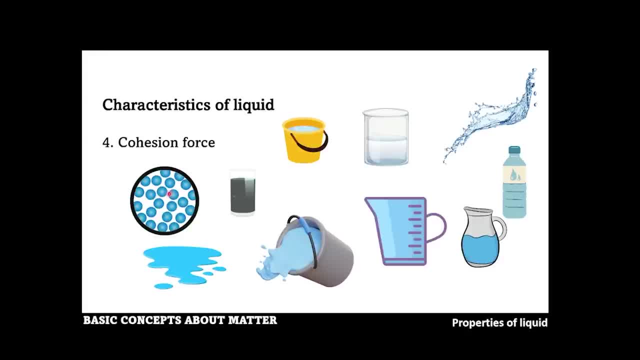 need to use the arrangement of the particles in liquid, because particle arrangement leads to different properties or characteristics of the physical state of matter. You will notice that the particles differ from what we saw under solid. The particles of solid are closely packed together, but the arrangement of particles 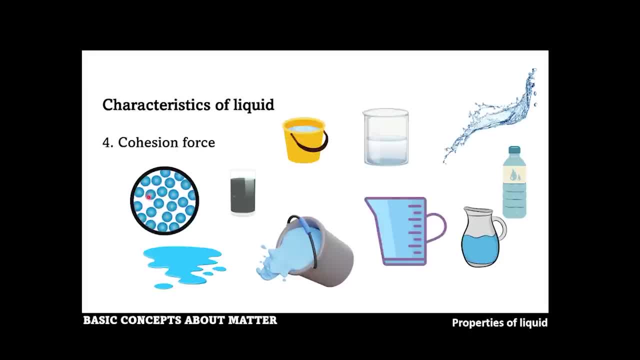 in the liquid has spaces between the particles and it is easy for one particle to replace another particle. The space between these particles of liquid occurs as a result of weak force of attraction between them. The particles are separated and they have weak force compared to solid. 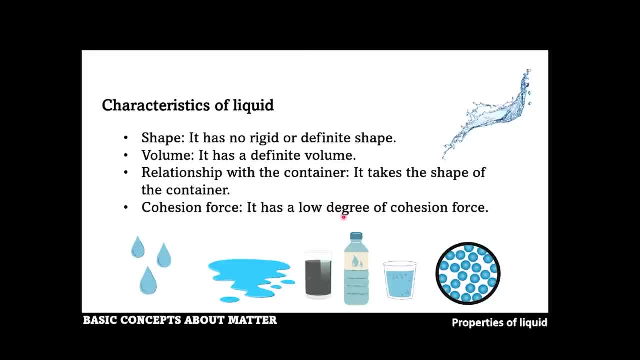 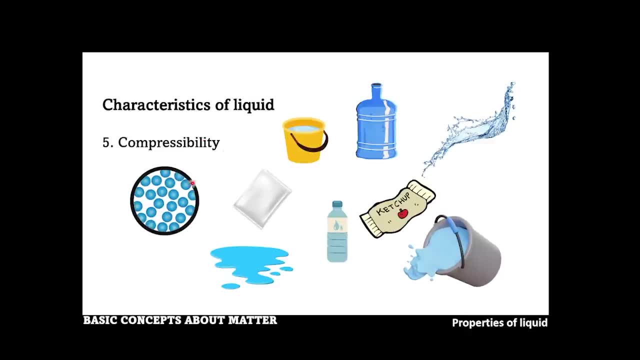 The conclusion is that liquid has a low degree of coercion force. The last property to consider for liquid is compressibility. Compressibility can also be understood by looking at the particles arrangement. The space around the liquid particles gives freedom of movement to those particles. 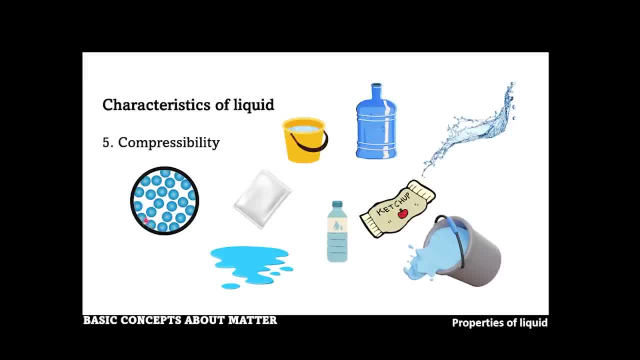 In that case, another particle can displace any particles or move to available empty space between the particles. When you press one side, the particles on one side can quickly move to the space available or replace another particle in its position. This is responsible for compressibility of liquid. 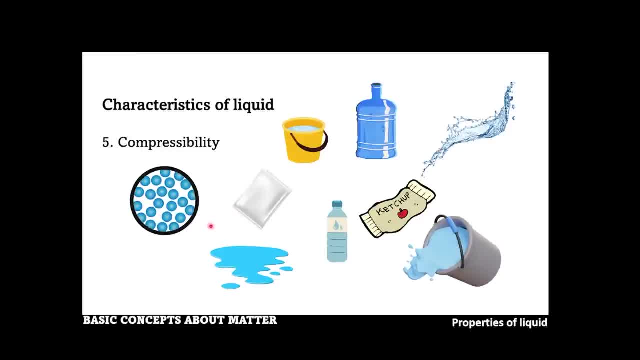 Let us look at the examples of items on this slide. The water inside the nylon, the ketchup inside the nylon and the water inside the bottle can be compressed because of the compressibility of liquid. When the liquid is pressed, the particles move to available space or replace other particles. 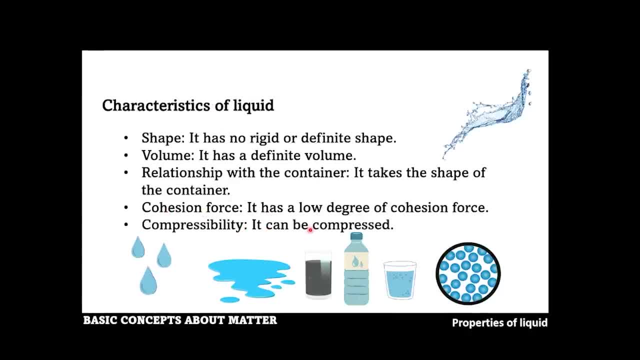 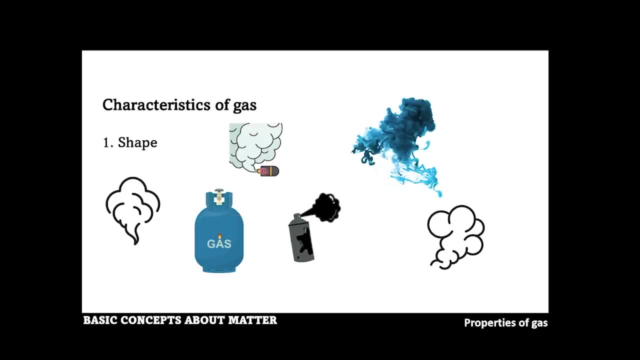 In that case, we can conclude that liquid can be compressed. That concludes the properties or characteristics of liquid. Let us look at the characteristics of natural gas. The gases are around us And many of them are colourless äng. However, even if we can see them when they are color gases, that is, those that are not colorless. 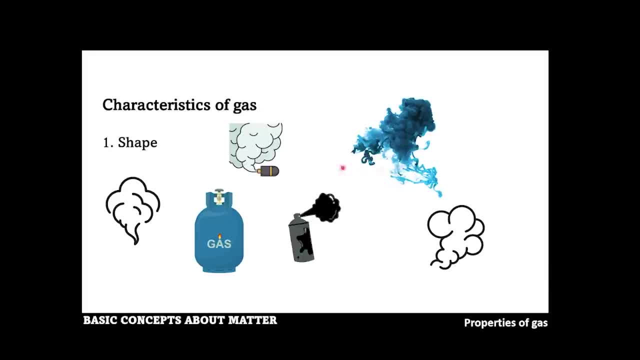 you will notice that they do not have a regular direction. Instead, they travel in what is called zigzag direction, that is, they move and travel without direction. If any gas is released into our atmosphere, there is no particular or specific shape to describe it. As you can see, when these 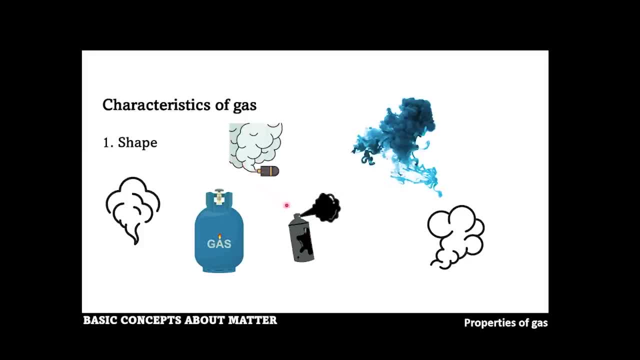 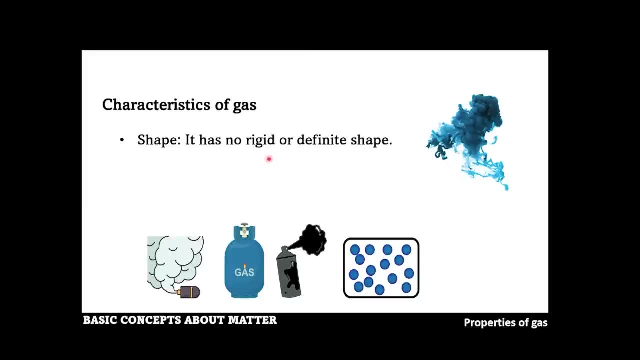 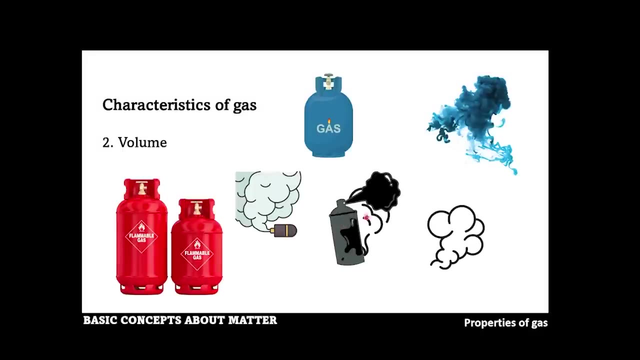 gases are inside the atmosphere, there is no specific shape to describe them. In that case, we can conclude that gas has no rigid or definite shape. In terms of volume, gas can fill different containers of different volumes. It does that by taking the volume of the container that holds it. Gas has the ability to fit into different 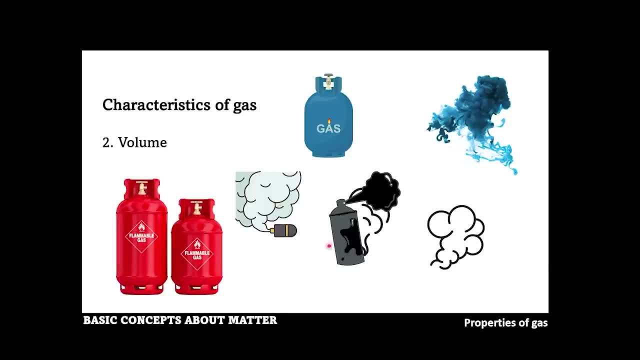 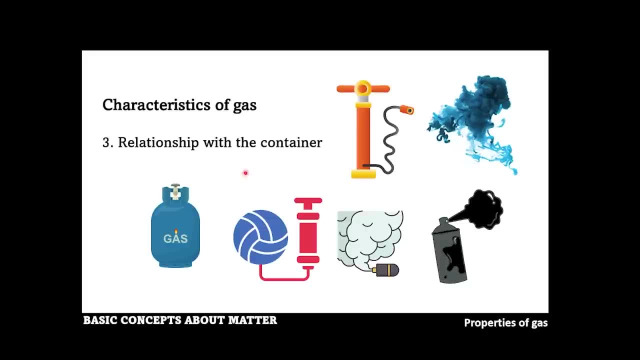 sizes of containers and fit in into different containers of different sizes, We can conclude that gas has an indefinite volume In terms of relationship with the container. gas also takes the shape of each container of different volumes, of different sizes. So the shape is detected by 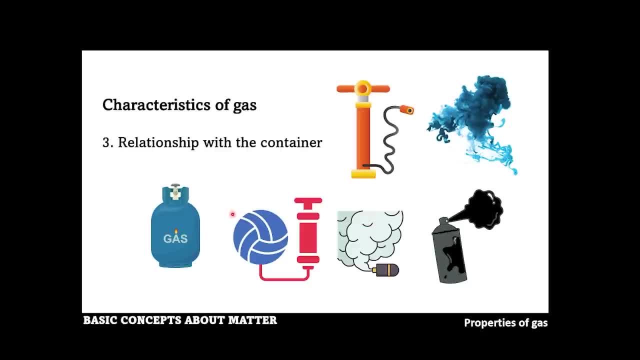 the type of container used to hold it. As you can see, when gas is in air, it can be described by the size of the container, and when it is inside this pump, it can be described by the size. The shape of gas is detected by the type of container used to hold it. 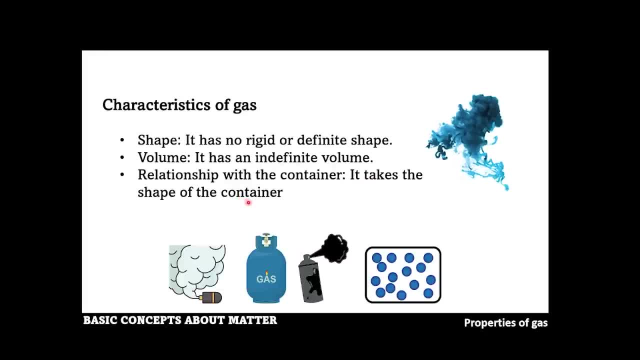 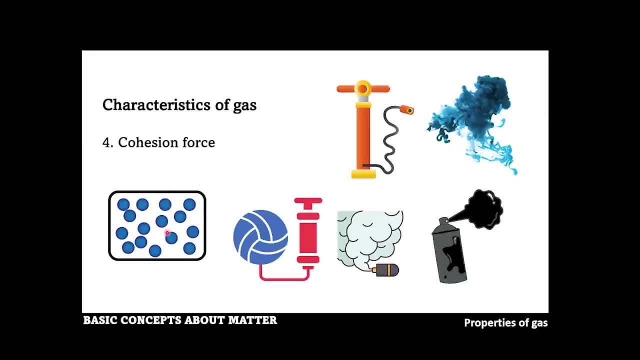 traumatic- define that kind of affair. this is practically the negative point that we can isolate in the air. In conclusion, gas takes the shape of the container, what is called cohesion force. The cohesion force of gas can also trace back to the arrangement of. 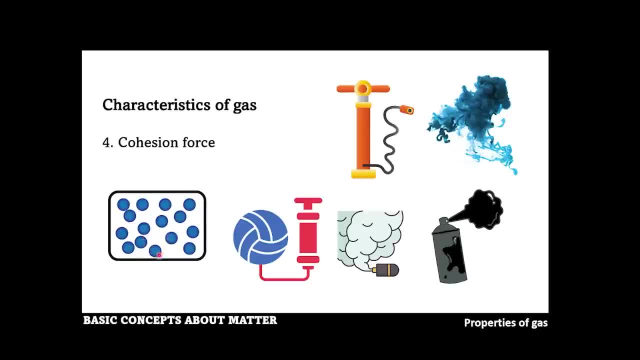 particles. Looking at the particles here, when you compare these particles to those in solid and liquid, you will discover the particles here are more spacious. This is responsible for behavior of gases. The space between the particles give them high degree of movement. The particles have 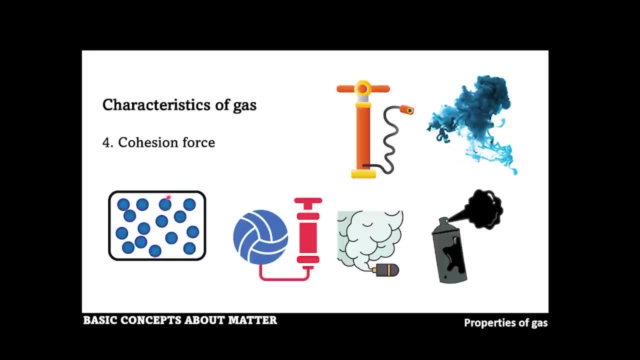 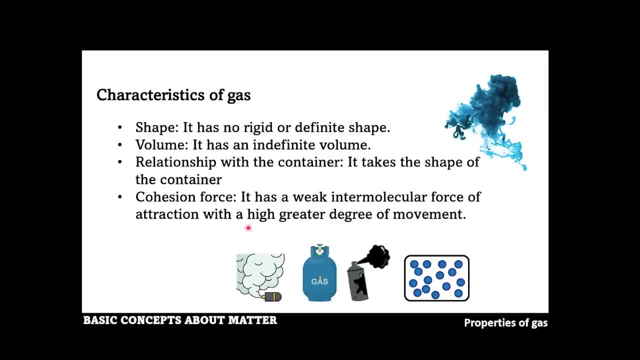 more spaces compared to that of liquid, and it is as a result of weak intermolecular force that exists between these particles. In that case, we can conclude that gas has a weak intermolecular force of attraction with high degree of movement, because those particles have enough space to displace one another and also move to empty spaces. 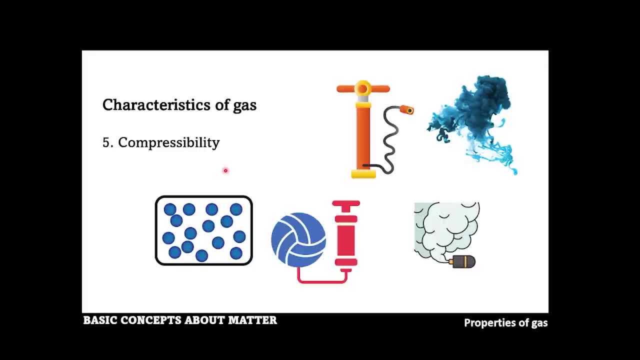 The last. This property is what is called compressibility. In terms of compressibility, it can also be explained using the particles arrangement. The particles have enough spaces to move and replace other particles or move to empty space. The ability to replace other particles or move to space leads to the compressibility. 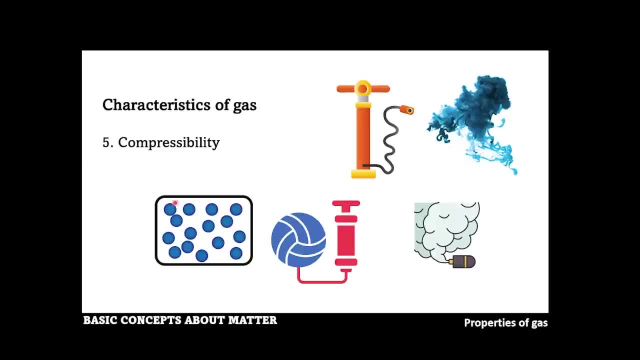 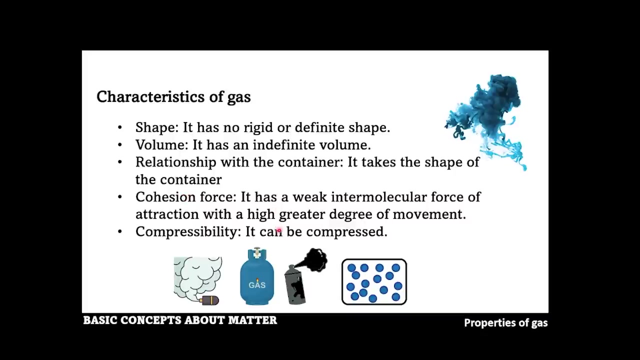 of gases. When a force is applied at any part of these particles, each particle can move to another space or displace another particle. It's as a result of the weak intermolecular force between the particles. In that case, we can conclude that, in terms of compressibility, gas can be compressed. 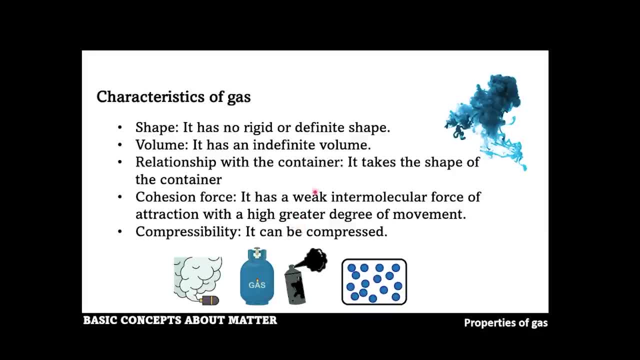 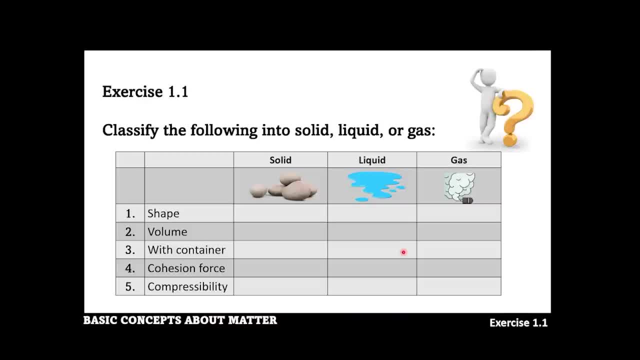 So these are the properties used to classify those items that I showed you. I have simple exercises for you. I want you to fill in the differences between solid liquid and gas. You will notice that they are everything that we've discussed so far. 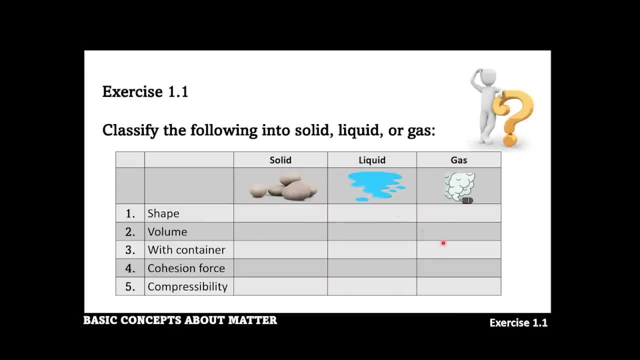 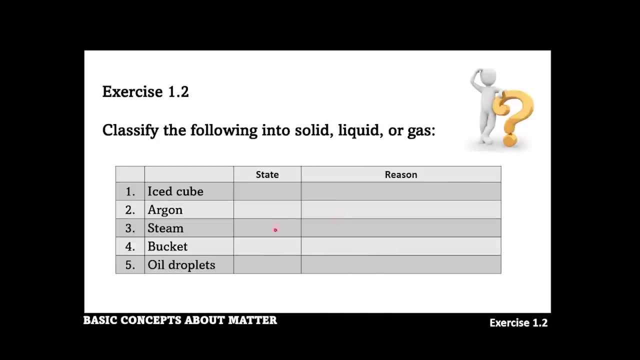 I want you to try it on your own and after you've tried it, you can check the solutions on our page. The second exercise: I want you to classify the following into solid liquid or gas And the next colon. I want you to give reasons why you've chosen that. your answer here is: 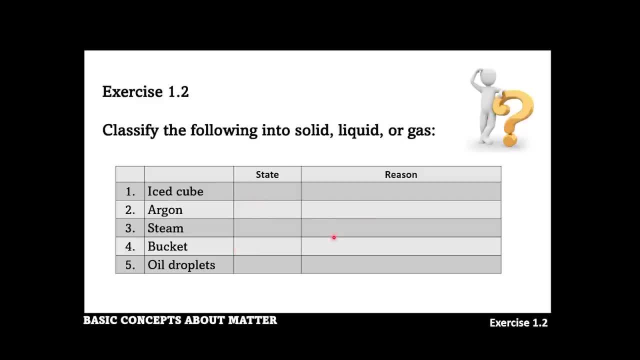 solid liquid or gas? As a science student, you must grow to a level where you question every decision you make. So by the time you classify them, I want you to give me the reason why you think it is a solid liquid or gas. 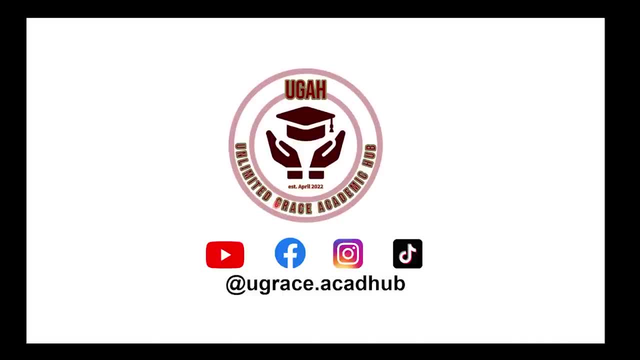 And that concludes The physical state of matter. In the next video I will discuss properties and changes in matter. Thank you for watching. See you in the next video. Bye for now.